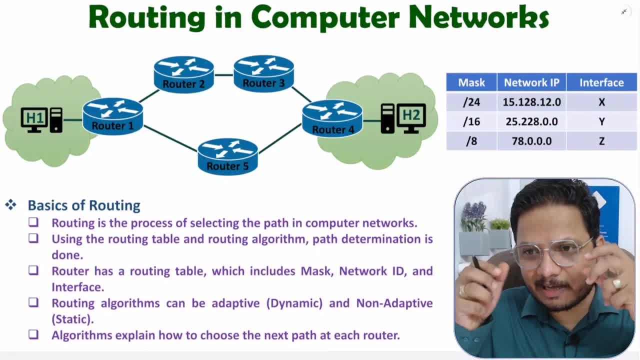 one device, then it is possible. if one device wants to forward frame to second device on internet, Then on internet there will be so many intermediary holes, So there can be so many paths by which that frame can reach from source to destination. So how many paths? 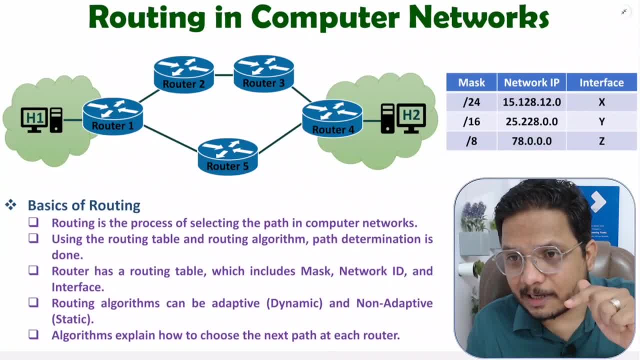 are there and out of those paths, which path will be selected? that will be defined by routing. So the end user has a variety of path types. So first of all let me give you one small example. Like, for example, if I say: here I'm having host one and here I'm having host. 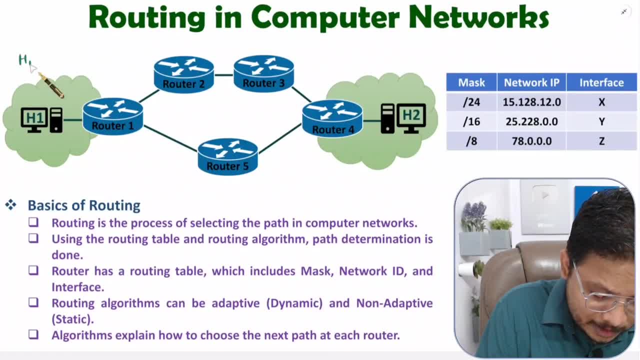 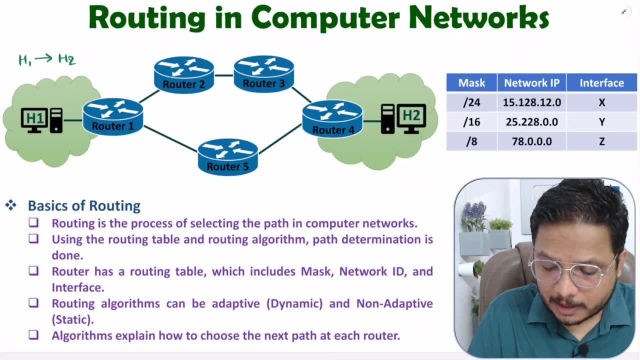 Let us say host1 is forwarding frame to host2.. So how that frame forwarding will happen, You see, here there can be multiple paths. First, host1 will be giving frame over here to router1.. Now you see, router1 is having two integer values. So I'm giving an integer. 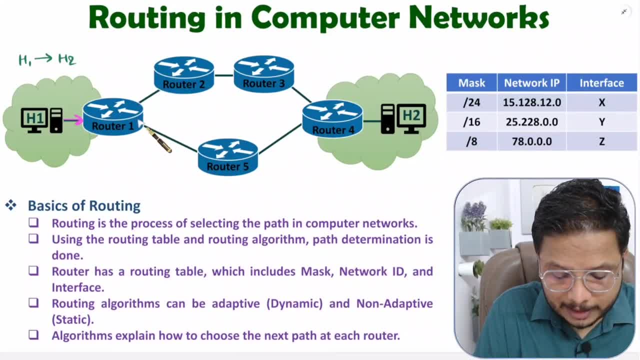 value as host1, and again I'm giving an integer value as host2.. So from here, whatever the parameter is, I'm giving an integer value. So I'm giving an integer value to this. Next here, this is one parameter that is been used for routing with an index. 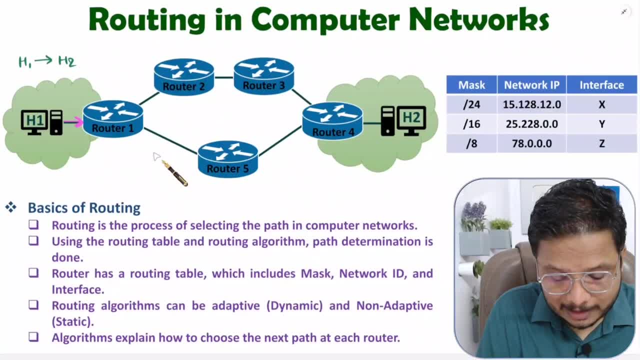 interface over here. One interface is connected with router 2 and second interface that is connected with router 5.. So here router 1 will take decision. That decision will be there based on algorithm, But router 1 will take decision to forward frame in this direction. It may forward. 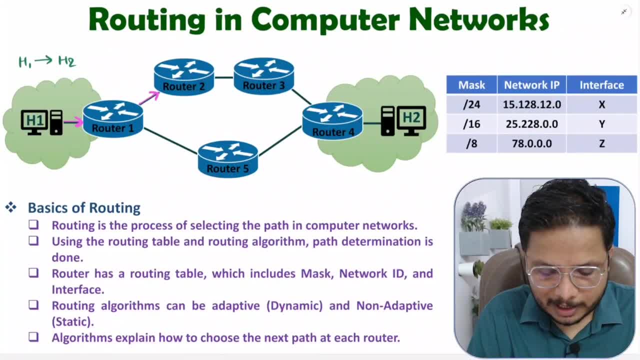 frame over here. also. That depends on algorithm. Let us say it is forwarding it over here, Then router 2, router 2 is just connected over here. So router 2 will forward frame over here and router 3 will forward frame over here, And once this frame reaches to router 4, router 4 knows Okay. 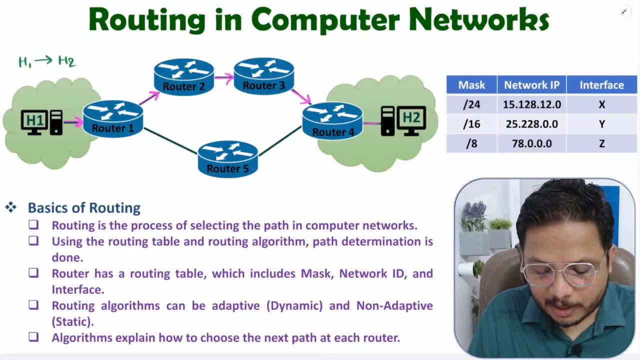 Here I am having destination device. It will give frame over here, Right? So see, router 1 knows h1 is connected here And router 4 only knows h2 is connected here. Otherwise, other routers are not having an idea about where is h1 and h2.. Remember this. So here how this path is getting. 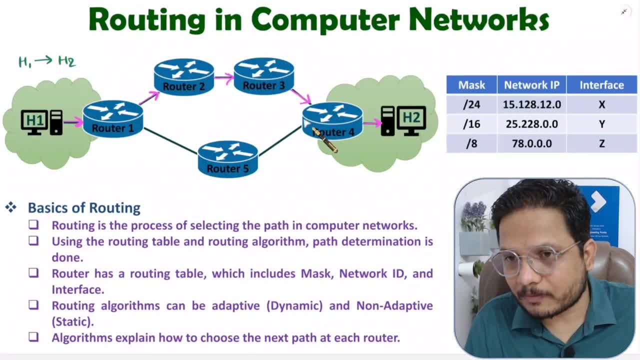 determined Right. That is referred as routing. Now, here, you should know, with router there will be tables, And standard format is like this: only In which there will be mask. After that there will be network IP And, based on network IP, there will be interface. Like you see, for example, if I talk about 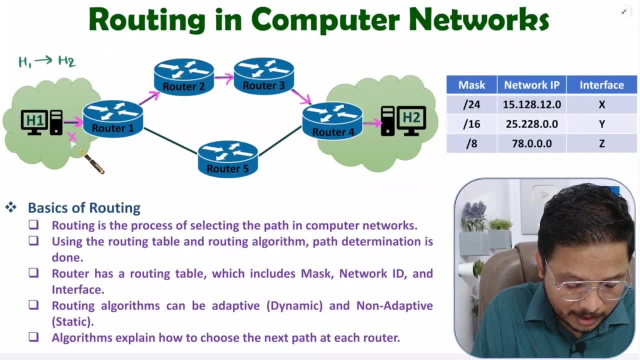 router 1.. So router 1 is having interface x over here, Router 1 is having interface y over here And router 1 is having interface z over here. So what router will do? Router will see frames over here, Which is having interface x Now, as if frame comes over here. After that it will. router 1 will. 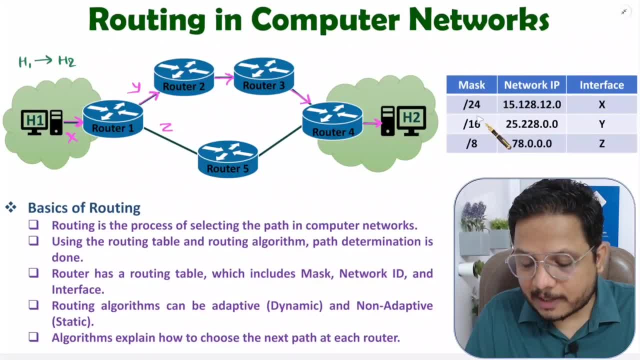 do masking. So let us say it is doing masking in sequence. So obviously frame comes from x, So it will not check for x, But it will. it will check for now y, So it will mask first After masking. if network IP is this, Then it will forward frame to y After masking, After masking, if network IP is. 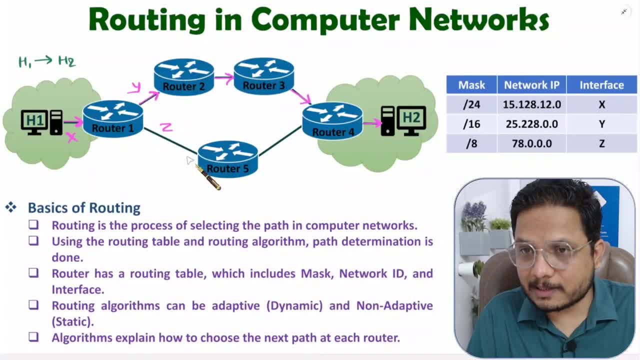 this, Then it will forward frame to z. See, this is how router is forwarding frames. So there will be table, So whatever destination IP is there, Based on that, masking happens And from masking it will be forwarding frames to interface. Interface means links, Right? So here, 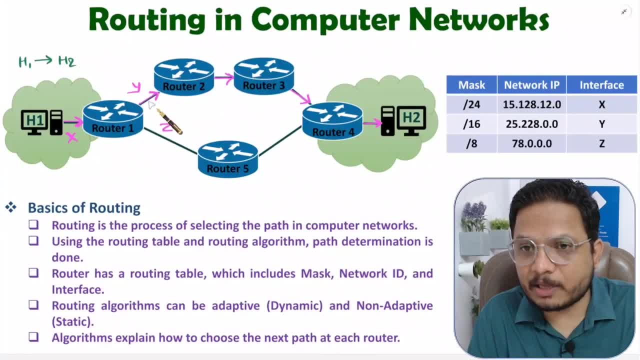 I have just shown you one example in which x to y forwarding is happening over. here Means from X frame is coming, Router 1 is forwarding it to y And this entries in table. that depends on how algorithms are there with this routers, So this router will be communicating with each other. 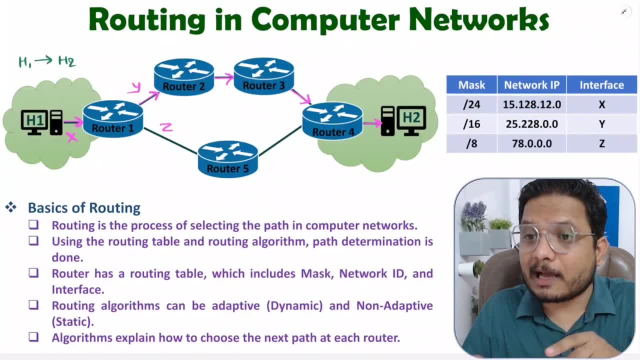 Based on algorithm, And algorithm will decide, like how frames will be routed in computer network. So let us discuss first how many basics are there. like you see here, routing is the process for selecting path in computer networks. using the routing table, routing algorithm, path determination is done. router has routing table which includes mask, network id and interface which we have. 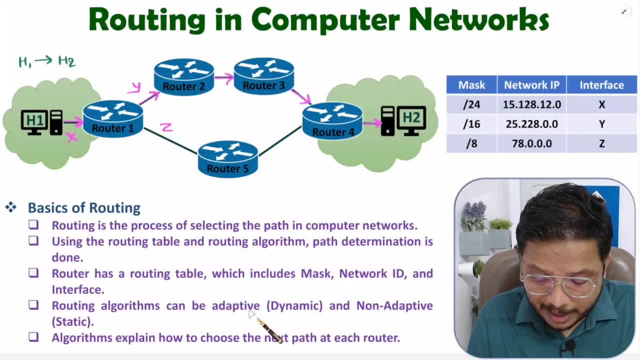 seen over here right routing algorithm can be adaptive or non-adaptive. adaptive means dynamic and non-adaptive means static. see, in dynamic path determination that will be dynamic, so that depends on parameters, and in non-adaptive path determination will be fixed. there will be fixed strategy by which path determination happens. in that non-adaptive. 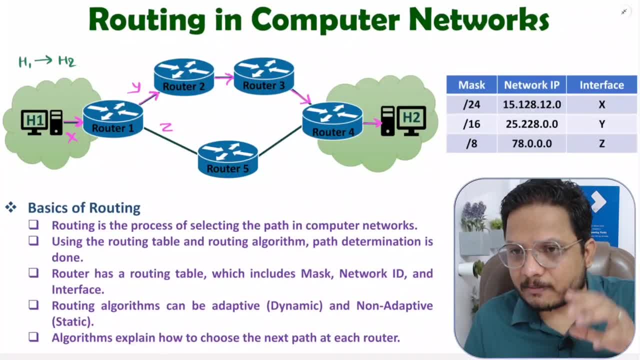 while in adaptive there will be dynamic strategies. right, I will show you what are the parameters, so that will give you more clarity. see algorithm explains how to determine the path of the router, to choose path from one router to other router. like you see here, when frame comes to router 1, then router 1 will decide whether to forward to router 2 or router 5. 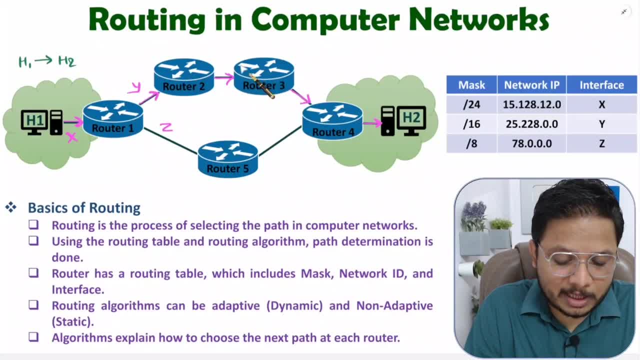 right. router 1 will not decide how to have communication over here at router 3 side. remember this. router 1 can decide only one thing: whether to forward frame over here or here. it may be connected with 3 interface, so it will have to take decision right, but that decision may. 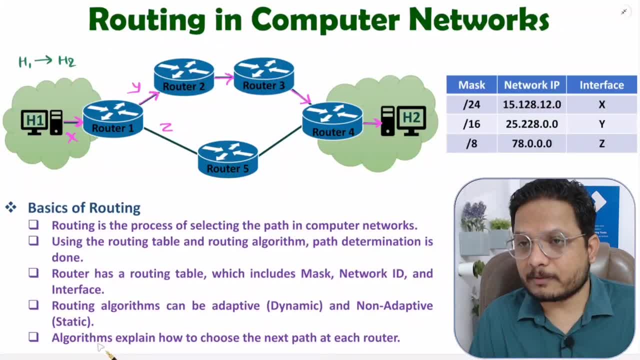 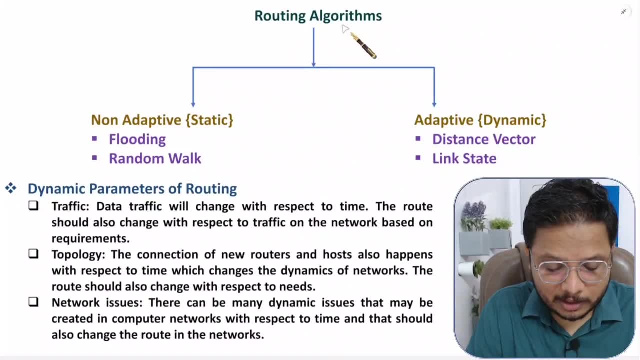 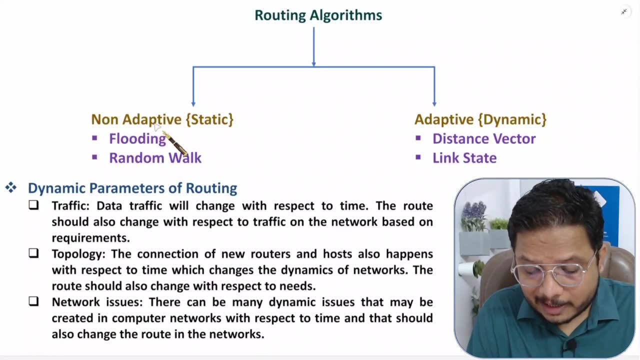 be that can be defined by algorithms. so let us try to understand how many types of algorithms are available. see, in general. there are two categories of algorithm. one is non-adaptive and second is adaptive. see, there are in category. there are two types, but in terms of number, 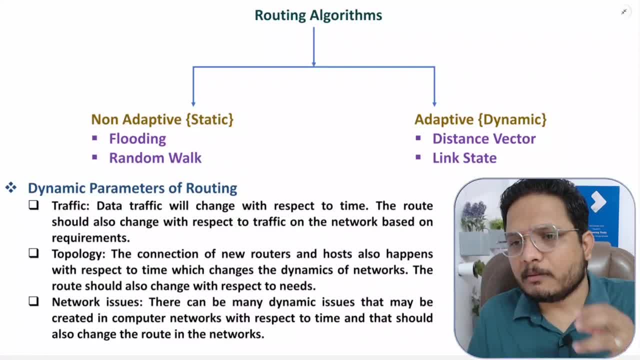 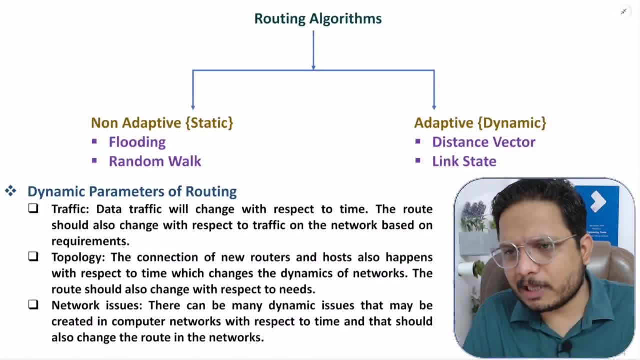 of algorithms. there can be thousands of algorithms. basically, in practice, I need to explain you this four. but there are so many algorithms available in the market right see in non-adaptive, widely used algorithms are flooding and random walk. see these two algorithms that I will explain. 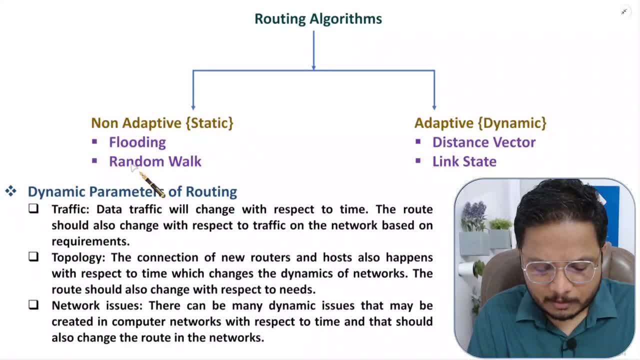 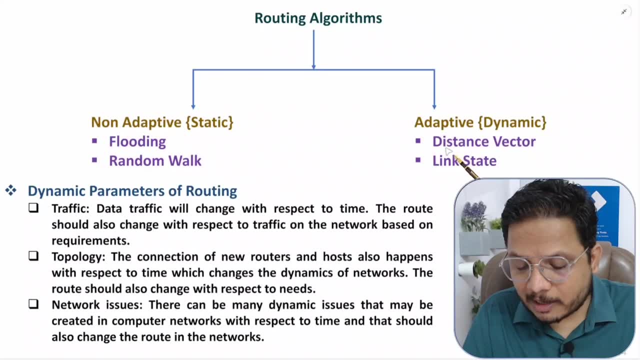 you in great detail right in next coming videos. but you need to understand these two algorithms are. non-adaptive means static and adaptive algorithms. those are distance vector and link state. see this link state algorithm that is broadly used right now. in 2023, in this entire. 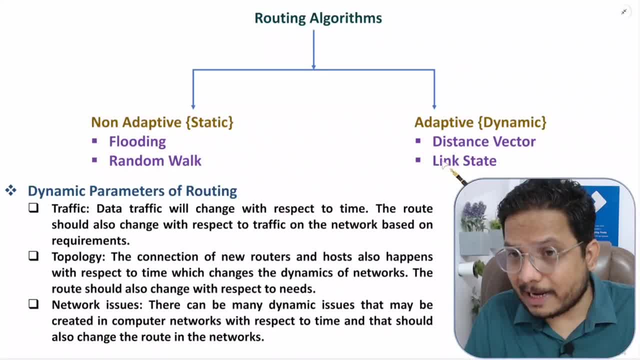 computer network. so link state algorithm that right now we are using right this distance vector algorithm that we were been using in 1990s and early 2000s. right now let me explain you how many dynamic parameters are there. see: static algorithm will not see this dynamic. 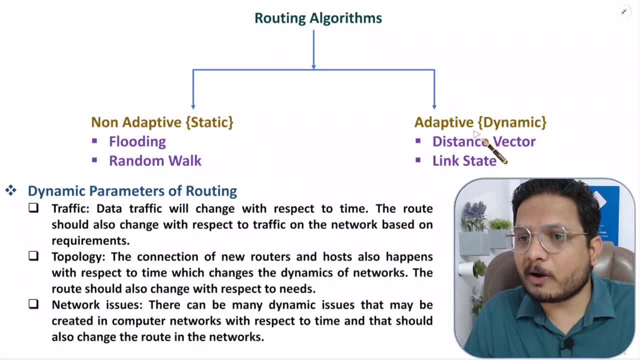 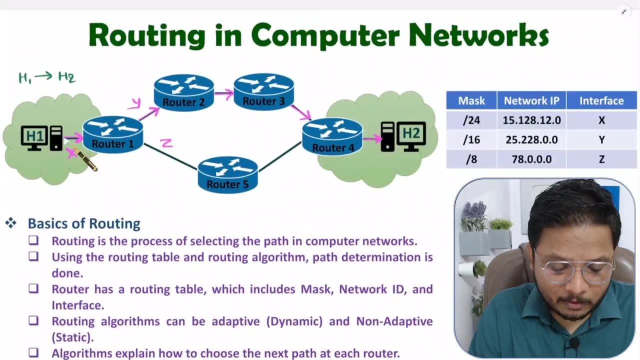 parameters. right, this adaptive algorithm will only see this dynamic parameters and, based on this dynamic parameters, it will take decision of router 1.. okay, see, those dynamic parameters can be traffic. see, for example, as if I say, here, here, right now, this path determination happens like this: but what if this router 3 is flooded by? so? 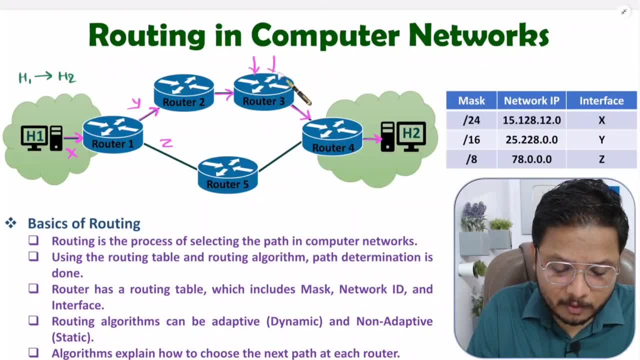 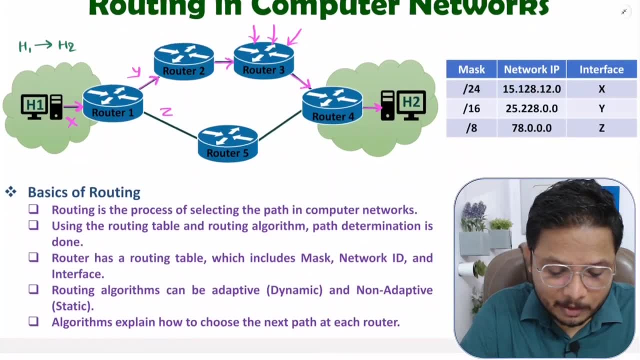 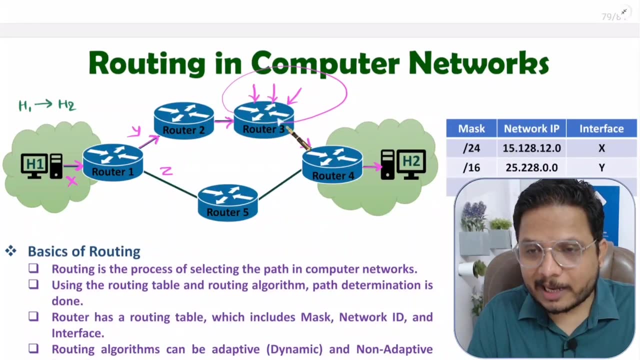 many data. what if so much data? what, what if so much data that comes over here like right, like see this router 3 that is also connected with some local area network over here, that is also connected with some local area network over here, like, if host of this local area network is forwarding so much data, then see, rather to 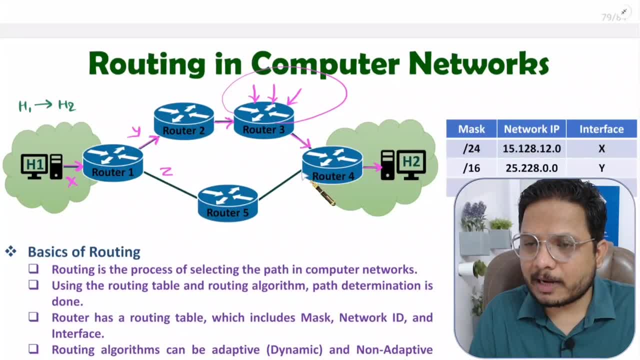 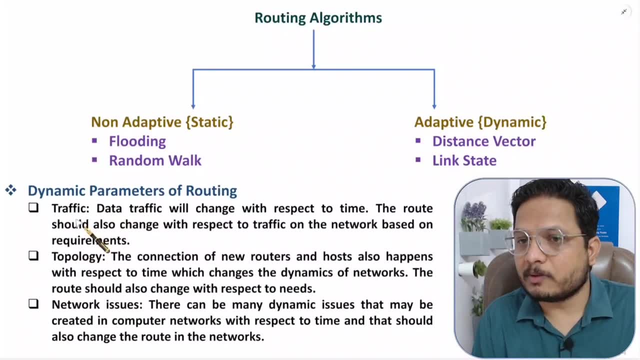 choose this path. this path is better, right, but that selection that can be done in adaptive algorithm only. so dynamic parameter is what traffic? so traffic will change with respect to time. for example, in your college, during college time, traffic at your college will be huge, but after college time period traffic will change. 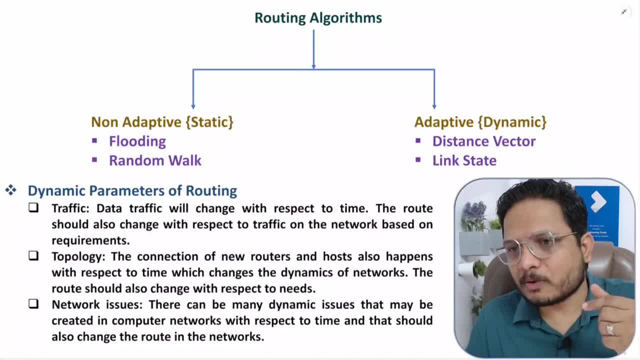 traffic will be very rare over there right. so at night time in the vicinity of your college, some homes will be there from where people are using internet. so at that time routing may happen via your college. but during day time, when students are there at your college, at that time traffic will be more at your college so other people will not be communicating. 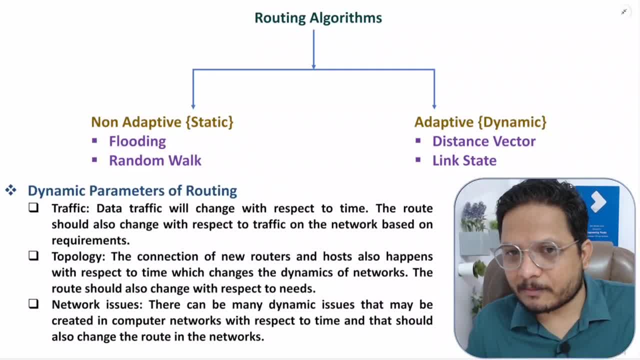 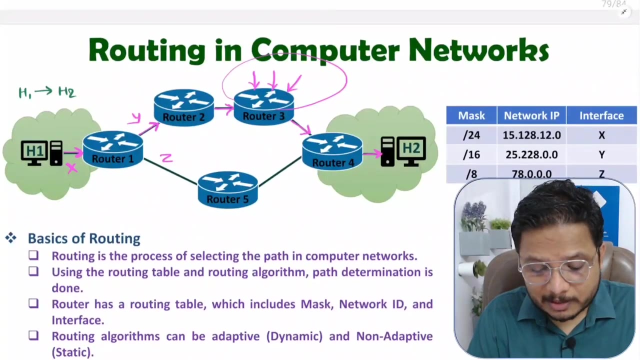 via your college. are you getting me see? this is how things are there. see topology also. dynamic parameter topology means so many devices may be connected in future. the reason is: see internet is flexible. many people are getting added, many people are getting out. that happens frequently. it is also possible, like some new routers may get connected over here. it is also possible.